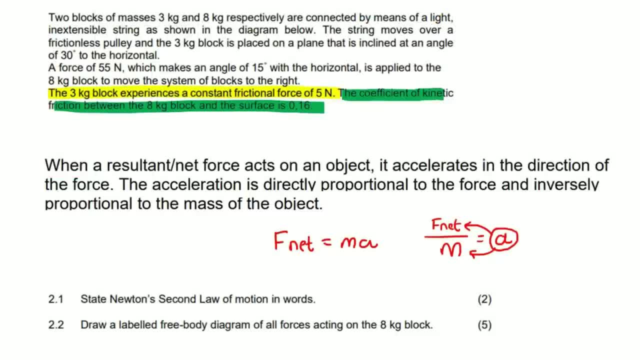 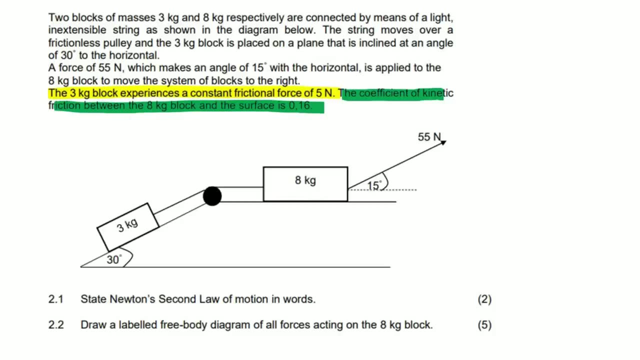 So there's the proper definition. When a resultant or a net force acts on an object, it accelerates. This acceleration is directly proportional to the force and inversely proportional to the mass. All right, so that's it. Next question: Draw a free body diagram of all the forces acting on the eight kilogram, And it's for. 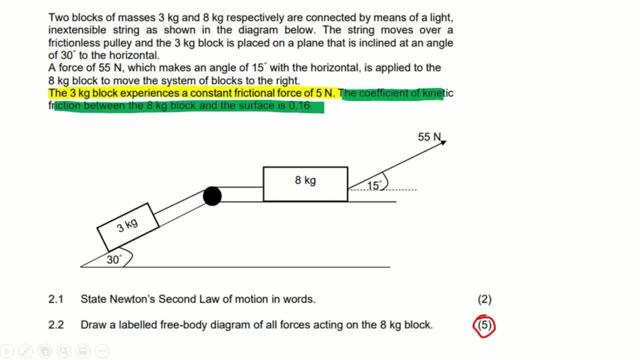 five marks. So that means we are going to have to look at five different things on that free body diagram. So let's put a little dot Now. there's always going to be a vertical gravity, So we can say f, g over there There's going to be a normal force, So we can say f? n, There's going to be a tension. 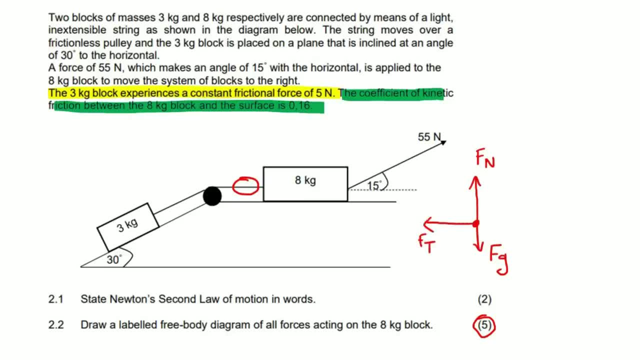 in this rope There's a frictional force. Oh, and that's important. Something I forgot to make mention of is that they tell us that the system of blocks moves to the right. Some of you might say, yeah, but can you tell us what the system of blocks is? 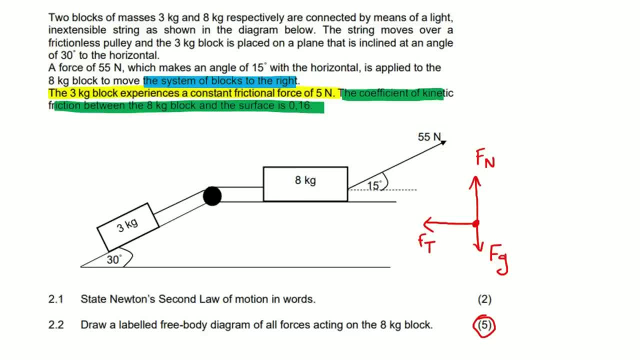 Well, Kevin, that's obvious because this arrow is pointing to the right. But that's not true. If this box is very heavy- let's say this box is 50 kilograms- then it could be heavy enough to cause this whole system to go down the slope, even though there is a 55 Newton trying to slow. 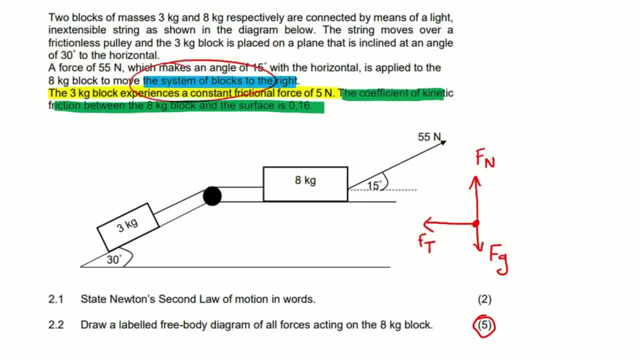 it down. So we do need to make sure about that. But here they tell us that we are going to the right, So we're going like that. Okay. so because of that we can say that there is a friction force in this direction over here. So I'm just going to say f like that. 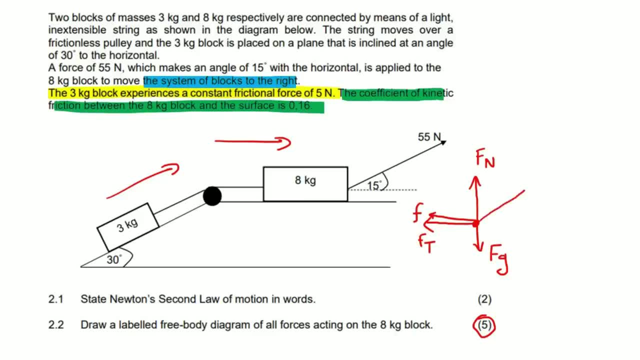 an applied force over here. so i'm just going to show it like that. and of course these aren't the only labels. um, for example, some, some, you're allowed to also use just n over here. for tension force, you can literally just say t, uh. for this one you can say w. for f, applied, you can literally 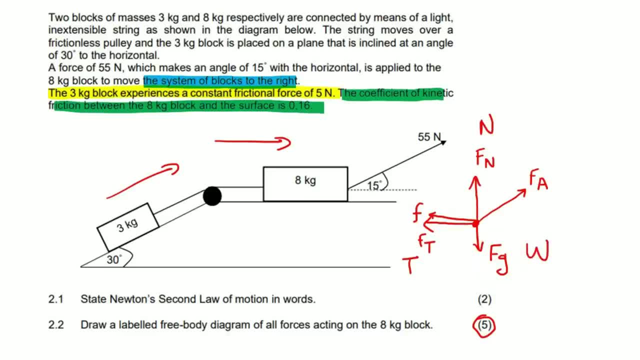 just say f, so they are different labels. okay. and then another thing is that some learners would prefer to break this up into components, and so what that would look like is the following: you would not have this one, and you would rather have um f in the x direction, and then you would. 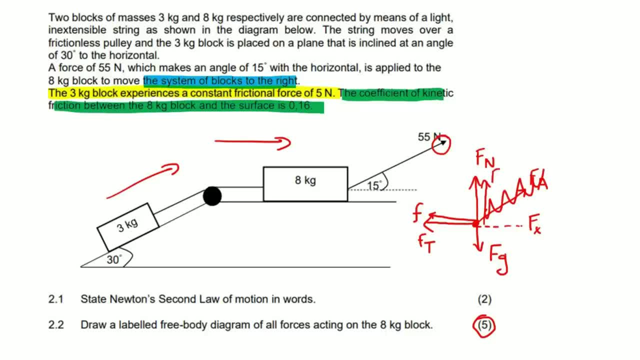 have an upwards force, because this one goes to the right and up and you would say f in the y direction. okay, but i don't like to use the component method. i mean, sometimes i do, i'm lying, sometimes i do do it, but i think for this one i'm just going to keep it as something like that. all right, so there's the. 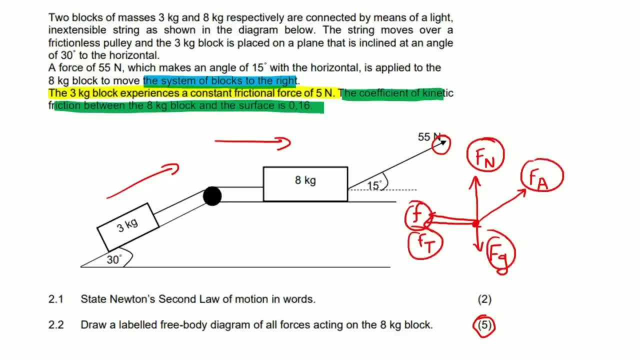 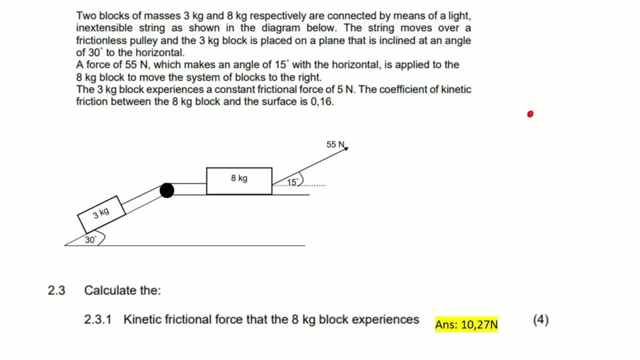 five marks: one, two, three, four, five. if you decided to break it up into components, then you can't say that that's going to be five and six. you only count one mark for all of that. i looked at this next question and i'm going to redo the free body diagram, but i'm rather going to use the components. 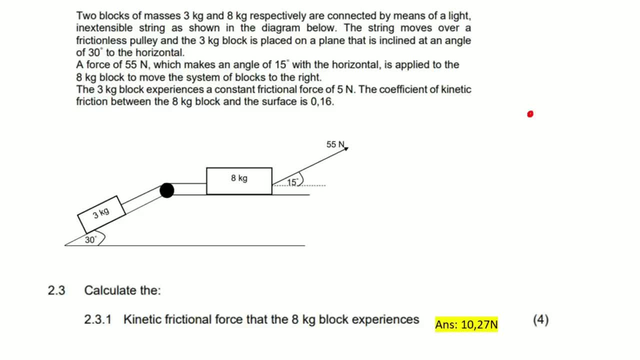 i actually do prefer using components. um, usually when it's on an incline- which for this one it is- i always use components. for this one, i sometimes use components, sometimes don't um, but i'm going to use components now, so we're going to have our normal force. 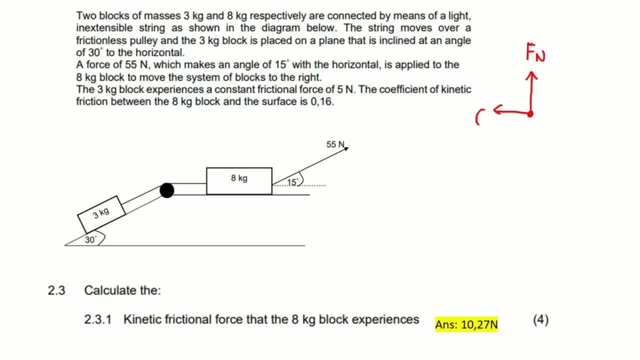 like we said just now, we're going to have our friction force, our tension force. some people just say t for tension. i'll actually just do it like that doesn't really matter. um, and then what else did we have? we had gravity, and then i'm going to use component forces for the force, so for force. 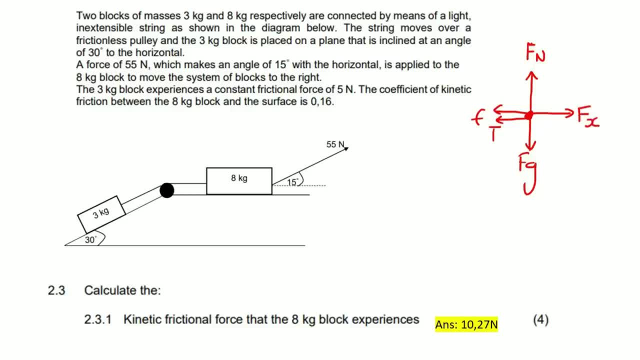 you can actually just say f, you can say fa, but i'm going to say f in the x direction and then f in the y direction. okay, so there's our different forces. now they want us to calculate the kinetic friction force for the eight kilogram. so we know that kinetic friction can be calculated using this. 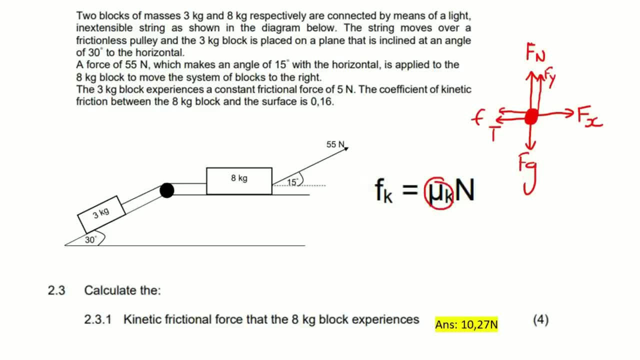 over here. so we need the coefficients, and they did give us that, highlighted it on the previous page, but they told us that the coefficient of friction for the eight kilogram is 0.16, so we already have this parameter. now a lot of learners make mistakes. 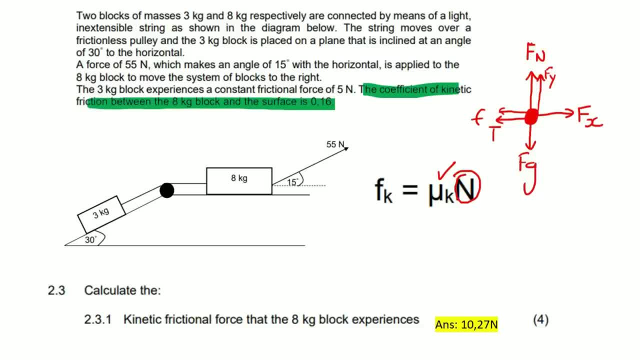 when it comes to normal force, they think that the normal force is always the same as gravity. that is only true if there are no other forces at an angle. as soon as there is a force at an angle, they are not the same, and i'll prove it to you by looking at your free body diagram. look at those. 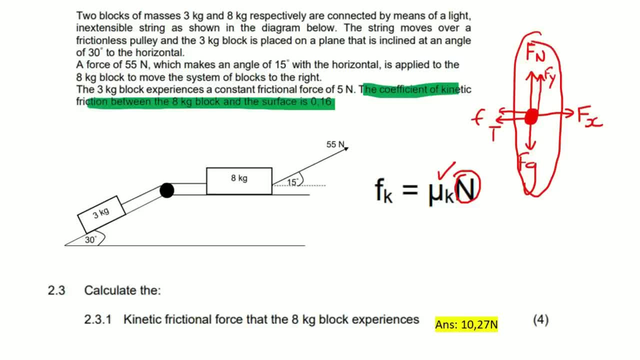 three forces they are all going to be. they need to be balanced so that the object doesn't go up and the object also doesn't go down. so these two forces going upwards, when you add them together they should be the same as the gravitational force. see that. 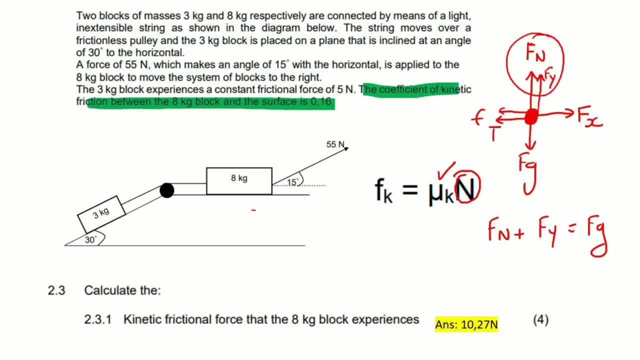 all the forces going upwards must be the same as all of the forces going downwards, so the normal force. we don't know what that is. if we had to work out the y component of this force, you would make a little triangle over here and this would be the y component over here. this. 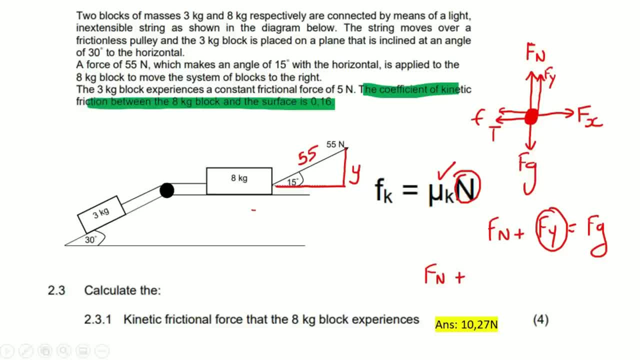 hypotenuse is 55 and so you would use the normal trigonometry like sin, cos or tan for that one over there. we're using this angle, we're looking for the opposite and we have the hypotenuse, so we're going to use sin, so you would say sin 15. 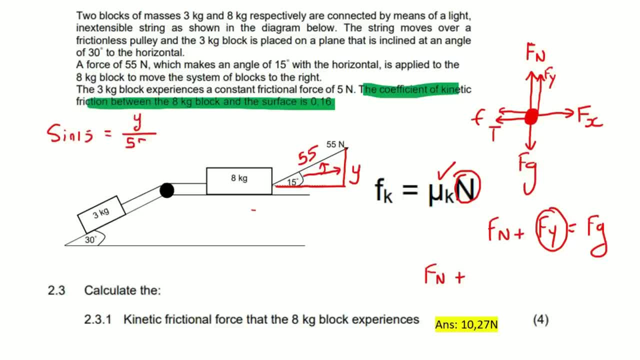 equals to the opposite over the hypotenuse. and if you had to work out y, it should be 55 multiplied by sin 15, and then i'm not going to round off. so that's going to be 14.2350. i'm going to keep four decimal places and we could say up, so i'm going to fill that in over here and then 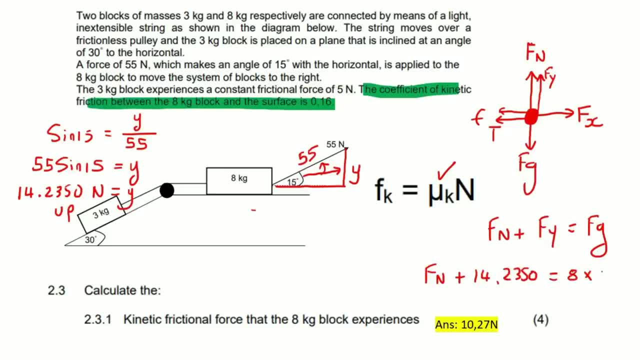 gravity is always the mass multiplied by gravity, which is 9.8. and so if you had to get the normal force, you should get the normal force, you should get the normal force, you should get the normal force and layer that from 1- socket to position one over. chuy Truly. 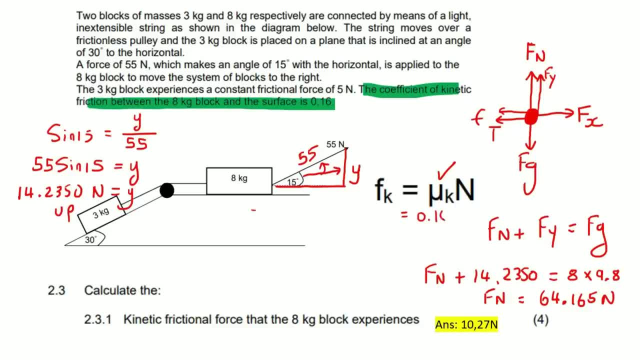 standardshaped formula. we would say: in this case you are going to get spinους stock in the height here. let's do the opposite, 64.165. i'm also not going to round off. so now i can use my friction formula and i can say the coefficient, which is 0.1. 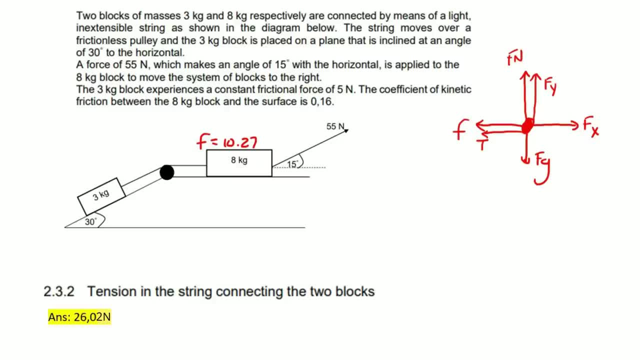 the next one or the last one says: determine the tension in the string. oh yes, and this one was for six marks. i forgot to write that one down, and i also wrote down the fact that the friction here, we now have that, and then the free body diagram, so it's very um well, actually, let's see. so this: 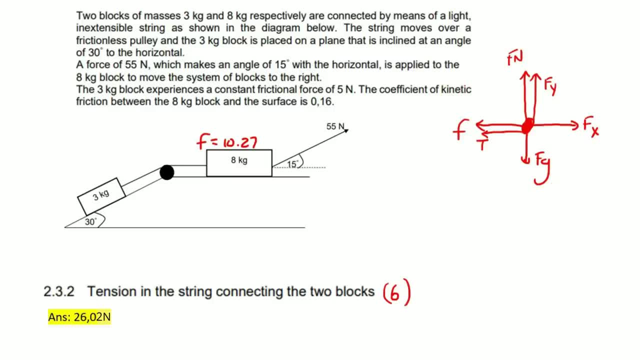 is the free body diagram of the three kilogram object. i mean, sorry, of the eight kilogram object. so if you've watched any of my videos with newton's second law, where we have two objects connected, you should know what i'm about to say. right now there are two unknown variables. 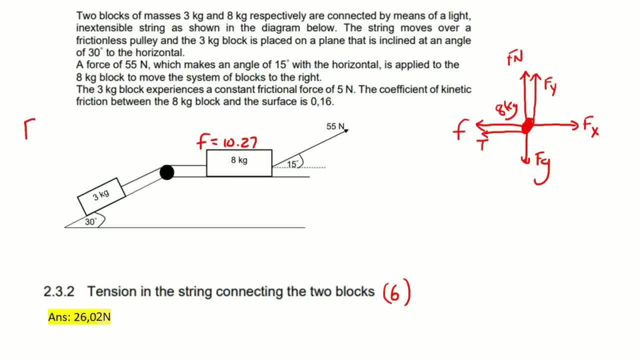 in this entire question, because if we use newton's second law, which is f net equals to ma, we know that all of these forces would go into the f net pot if we were only using this object right. so we, we know the friction, we know the x component of the force, but we wouldn't know the tension. so 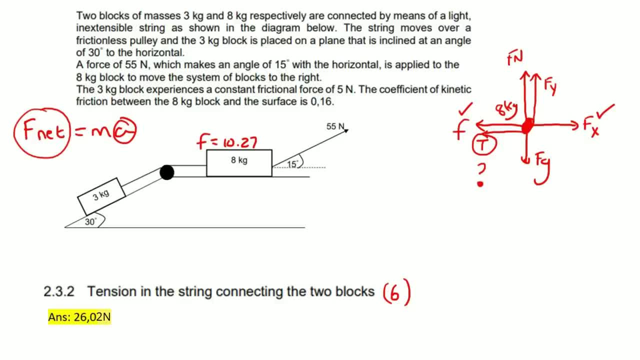 that's an unknown variable, and we also don't know the acceleration. they didn't tell us somewhere here that we're moving at a constant velocity or something like that. so we have two unknown variables. so, as i said, if you've watched any of my videos, we are about to do the same thing that we always do. and how does? 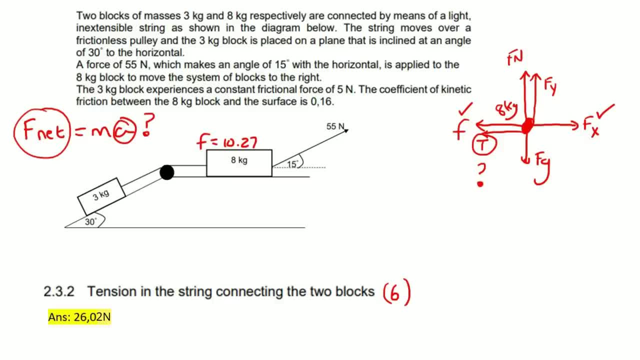 that go again. we make two free body diagrams of both objects. so let's do that quickly. we need to do a free body diagram for the three kilogram. so for the three kilogram it would have a normal force that would be the force of the three kilogram. so we would have a normal force that. 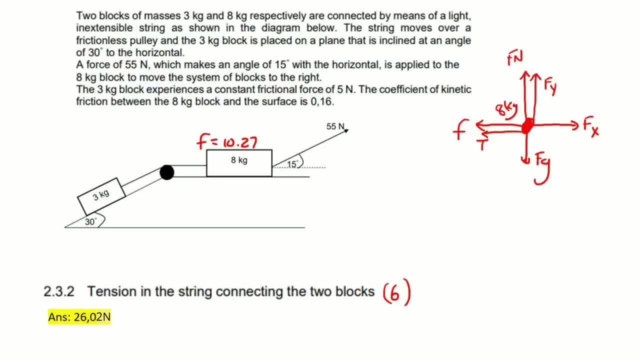 goes perpendicular to the surface, so i'm actually going to do it over here. so there would be a normal force going like this. there would be a tension in the rope going upwards, then there would be friction. they did tell us that there was friction. remember they said that the three kilogram 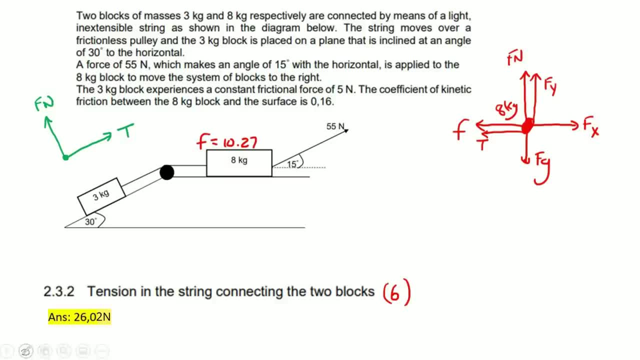 experiences are friction of five newtons, so we can do that now. what some learners would like to do now is they'll just put gravity going downwards like this, and then we're going to do the same thing. that, but if you've watched my lessons or if you see the way i do it, i like to use the component. 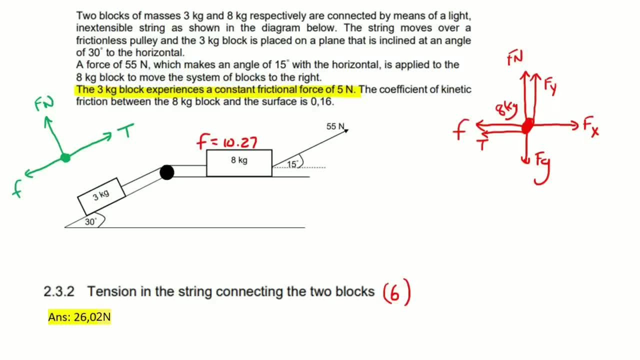 method instead. so i'd rather break up the gravity into its perpendicular component and its parallel component. why do i do that? it's just because it helps me with my calculations. it makes the calculations much easier to understand. so i'm going to use gravity perpendicular. so i'm going 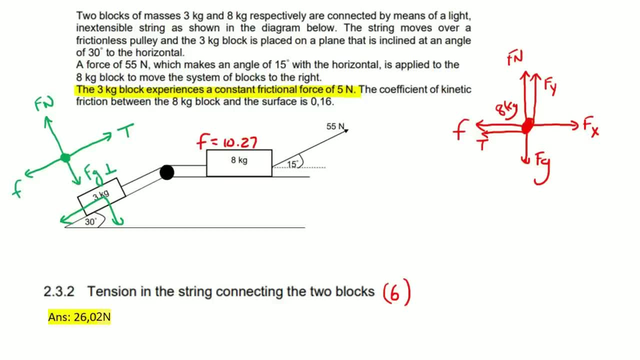 to say f, g, perpendicular, and then we're going to have a parallel gravity. people always ask me if parallel gravity sometimes acts up the slope. my answer is that it always acts down the slope, even if your object is moving downwards or if it's moving upwards, it doesn't make a difference. 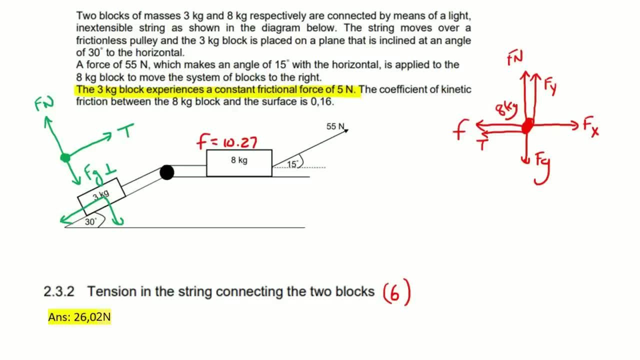 parallel gravity always acts down the slope. okay, so i'm just going to make the circle a little bit bigger so i can fit the friction and i can fit the. uh, what did we say? oh, f, g, parallel. right, so there we go. so what's our next step? so we do a free body diagram on both. 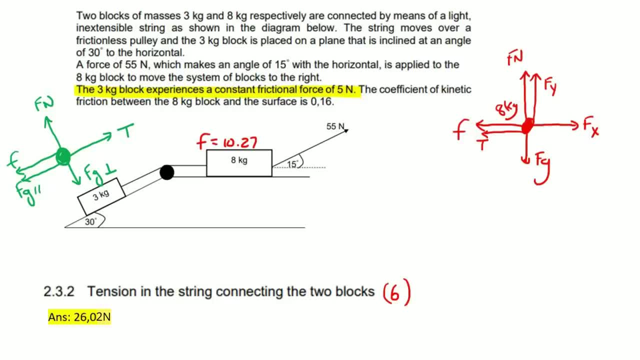 objects. we've now done that, which is great- then we're going to use f- net equals to ma- on both of those objects. so this is the part where i would then normally divide my page into two equal halves, and then i'll just do it for the three kilogram. 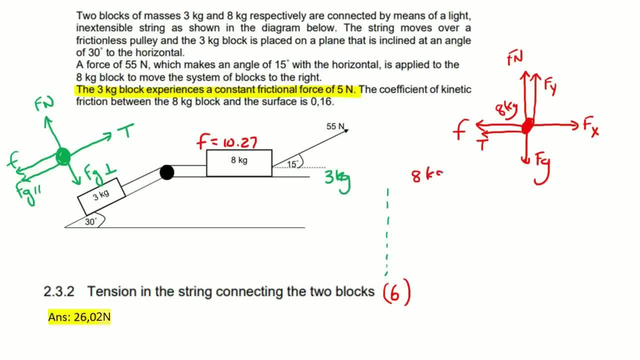 and for the eight kilogram, and i'd use f net equals to ma. so i'm going to go: f net equals to ma. and which direction do i want is positive? well, this is: we're looking at this object, so we're moving up the slope, like that. so i'm going to say up that slope, like that is positive. 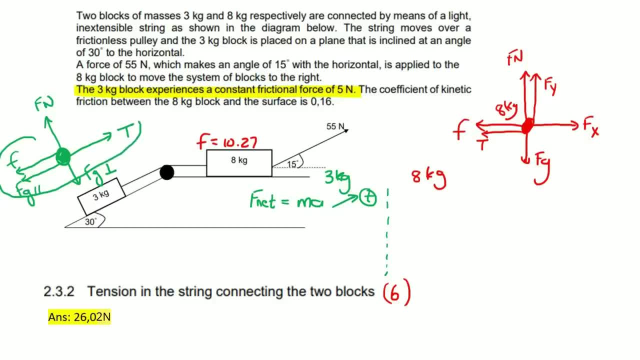 and then i just look at all the forces in the in the slopes direction. there they are. this is why i don't like to use gravity as going down. i rather like to use the components, because then i can just say that these are the three forces that i need to use. so all i literally say now is: i can. 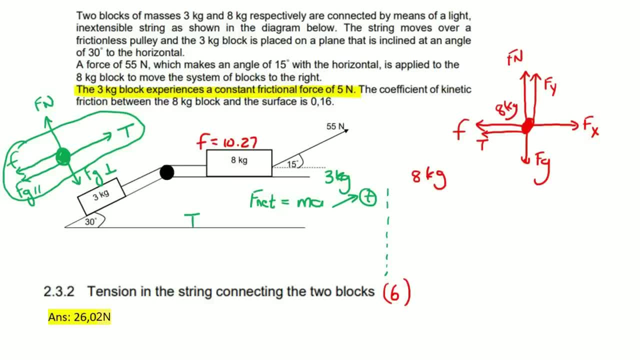 say tension force, which is positive because it's acting up the slope, minus friction, minus fg, parallel- how easy is that? because these are the three forces that we're looking at, and then i just make that equal to ma, then i go full in as much as i can. so the tension, i don't. 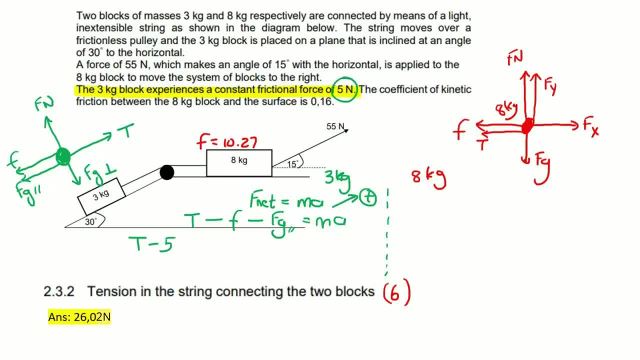 know, the friction force on that object is five gravity parallel. remember the formula for gravity parallel is mg sin theta. so i'm going to say minus three kilograms times 9.8, times sin of the slope, which is sin of 30, equals to 3a. so the two unknowns, as per normal, is going to be the t. 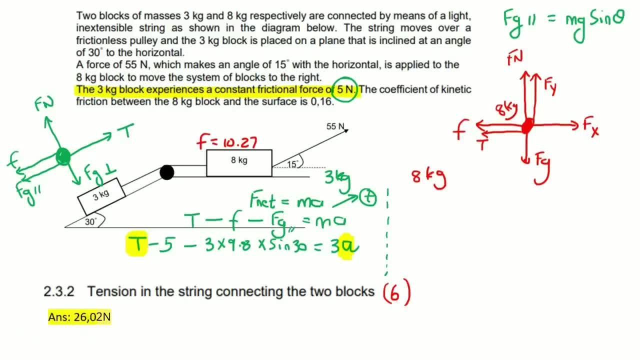 and the a. i'm just going to neaten everything up a little bit. so what i'm going to do is i'm going to put all of these together, so it's minus 5, minus 3 times 9.8, times sin 30, so that's minus. 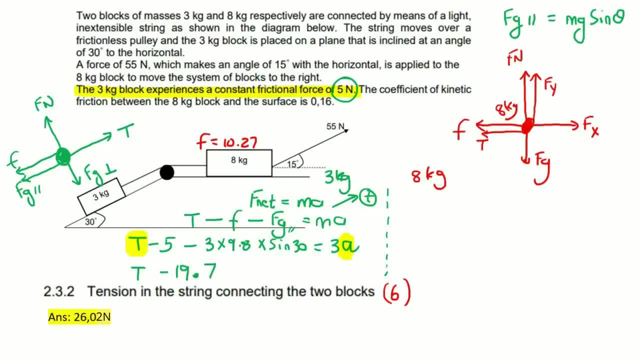 19.8, 0.7, and that's equal to 3a. so there's our first equation. we can't go any further. now we're going to go do the exact same thing with f net equals to ma. i mean sorry, with the eight kilogram. 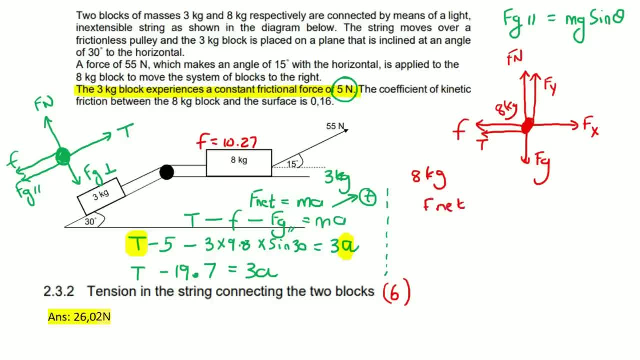 so here we're going to say: f net equals to ma. now this object's going like that. so i'm going to say: right is positive. and now it's so easy. look at my free body diagram. i just, i just use those three forces, but if you had some weird force at an angle here, then it's weird, right. so that's why i. 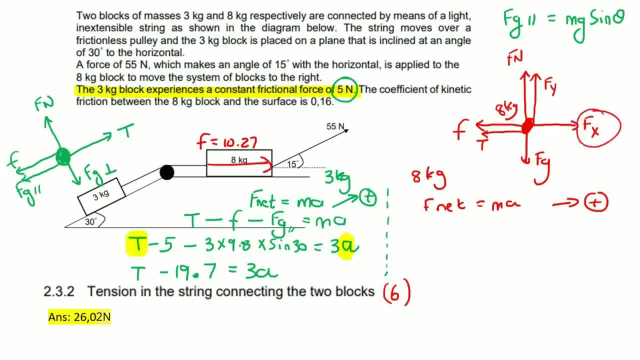 didn't use the x component because i now know that i just need to use the x component. so i'm going to say fx because that's positive, minus the friction force, minus the tension force, because they are acting in the negative direction. some of you are like, yeah, but kevin, in this one you said tension. 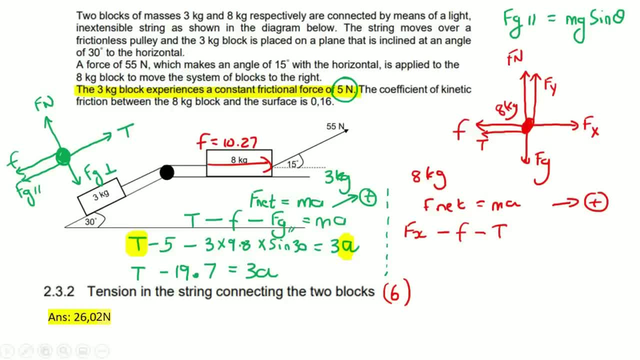 was positive, bro. yeah, but for different objects tension can make the thing go faster, and for other objects it can make it go slower. okay, so, and then we're going to make that equal to ma. there we go. so if we're looking for the x component, we need to go use trigonometry here. 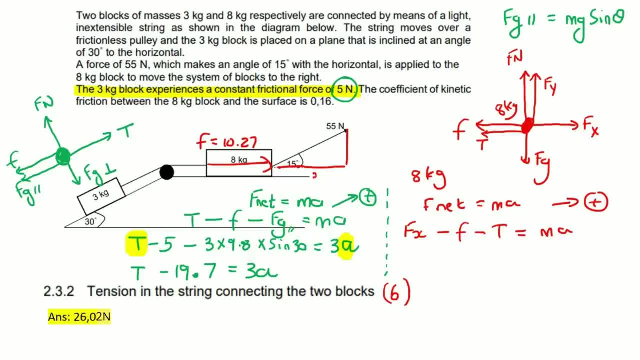 so if we're looking for the x component and we know the hypotenuse, then we would use cos. so we would say cos 15 equals to the adjacent, which is x over 55, and if you had to get x by itself you would get 55 cos 15. and if you had to work that out, i'm going to keep three uh. 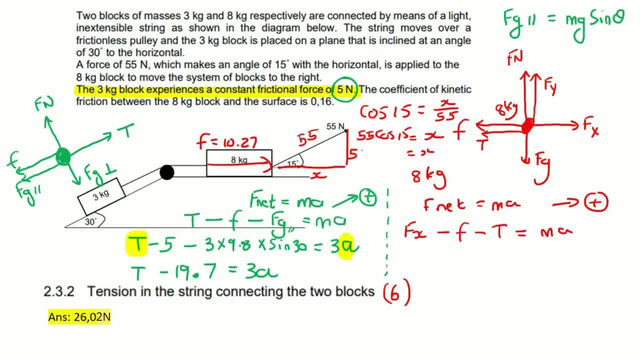 four decimal, sorry. so that's going to give us 53.1259, okay, and you could say to the right and then: yep, that's it. so we're going to say 53.1259 minus the friction force that we calculated earlier, which was 10.27, minus tension, which we don't know equals to the mass. 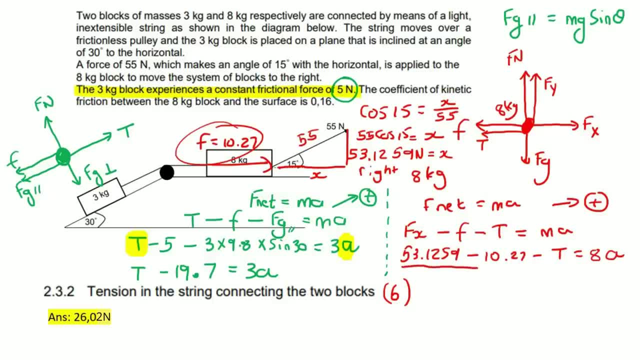 of that object, which is 8 and a. what i'm going to do now is just put these two numbers together, not going to round off. so that's 42.8559 minus t equals 8a, and there's our second equation. so now we're just going to link this one and this one simultaneously. now you can do that, however. 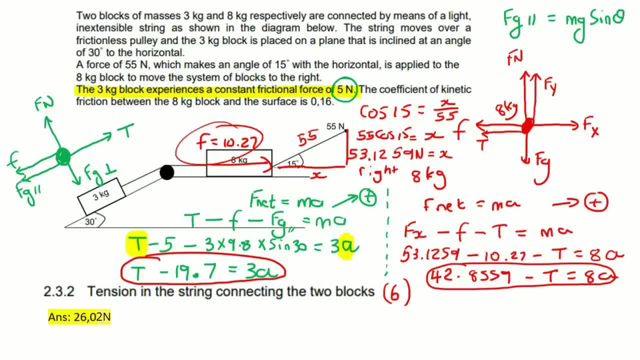 you like. what some learners like to do is they like to get the tension forces by itself for both of them, to make the two equations equal. but then what other learners like to do is they rather they get one of them by itself, like they'll get this one by itself and then they'll plug that into. 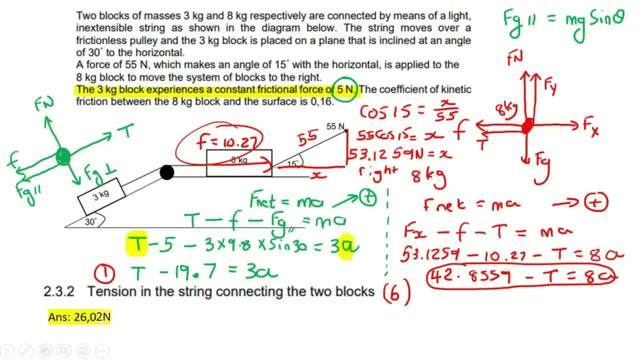 this one. it doesn't matter. you do whatever you like if you're comfortable with with simultaneous, but obviously we must get the same answers at the end. so what i'm going to do is i'm going to take this one and i'm going to get the t by itself. so, for example, if this is equation number, 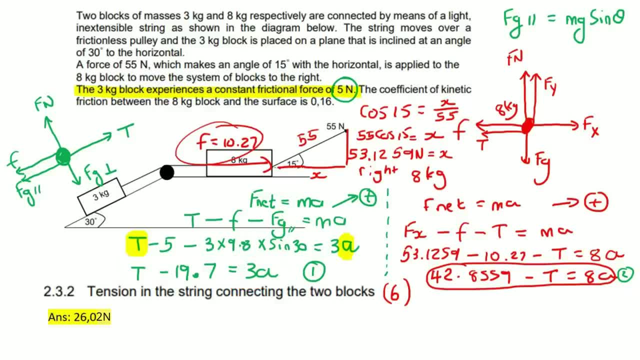 one. this is equation number two. i'm going to quickly rearrange equation number one to become: t equals to 3a plus 19.7, and then i can call that number three, and then i'm going to substitute number three into number two. so i'm going to sub three into two, so we're going to end up with 42.8559. 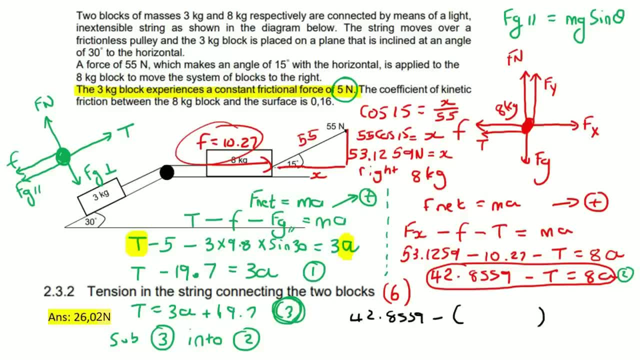 minus, then please, please, please, use brackets, because, especially that minus, it's going to make things wrong if you don't use brackets. so then you're going to say 3a plus 19.7 plus 19.7 and that's going to be equal to 8 a. you see, now we only have a's. 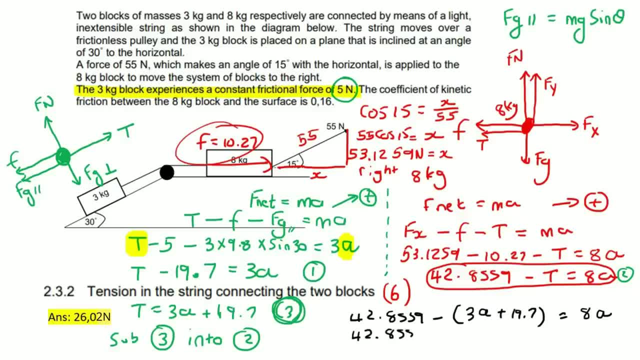 and so then we can say 42.8559 minus 3a minus 19.7. a lot of learners will get that part wrong because they don't put a bracket, so it becomes plus 19.7. so if that's what you're doing, don't. 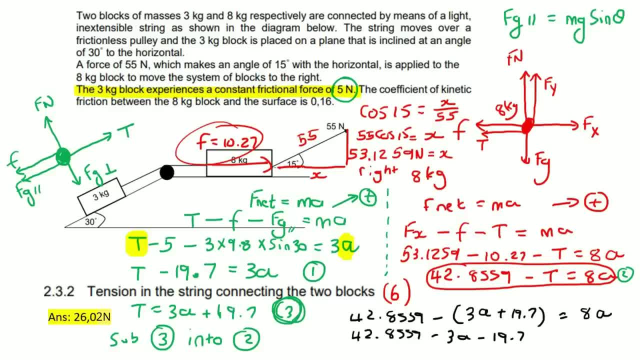 worry. it's a small mistake, but it is a very popular mistake. it's something that i see a lot ofaut enjoying. so now we can do 3a over half here, so we have that equal to 8a, that's equal to, that's equal to 8a, and so now i'm just gonna carry on up here, so i'm gonna minus these two values.